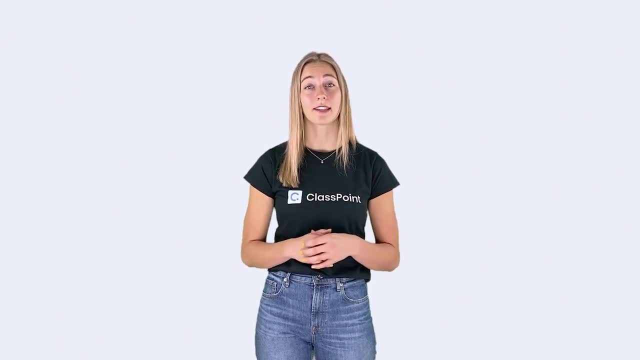 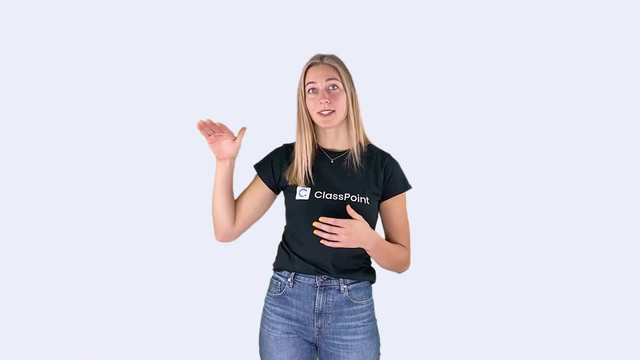 There are endless ways and opportunities to add gamification into your class, but today we're just going to cover the four most popular, And the good news is you can pick and choose. You can keep it simple, stay surface level or deep, dive into any of these aspects. 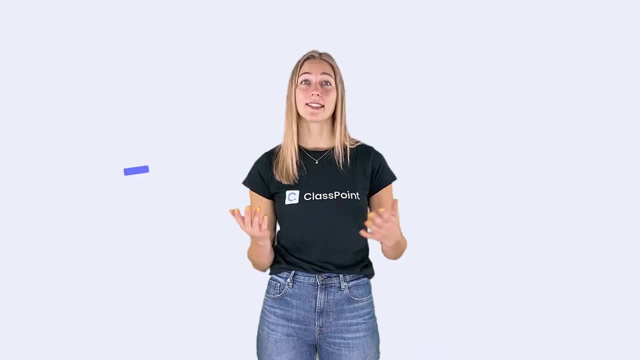 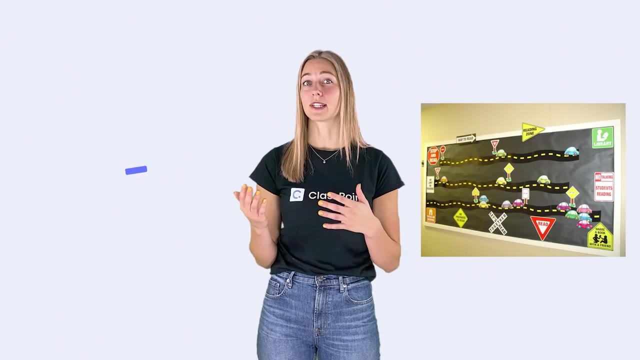 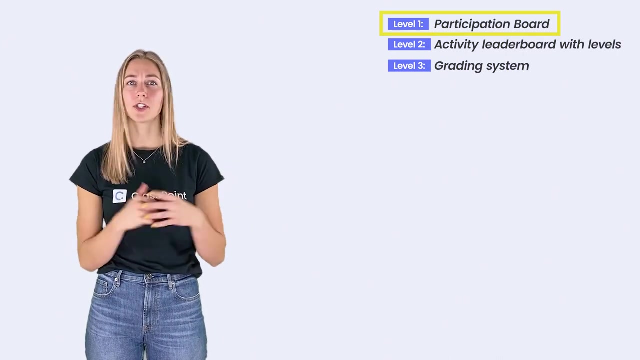 Do what fits best for your classroom. Start out easy with a point system and a student leaderboard So you can turn those daily activities into student progress boards. or you can take it a couple steps further and completely change your grading system. The first level of this is just doing a simple participation board. Points can 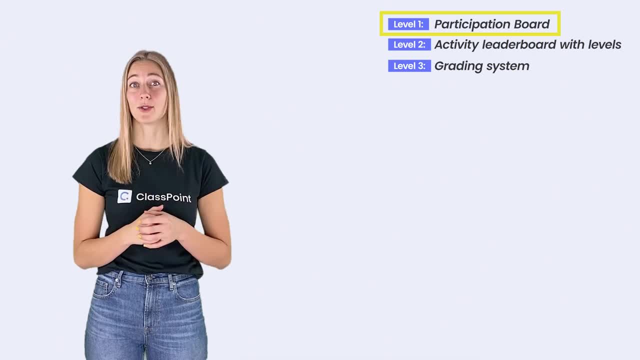 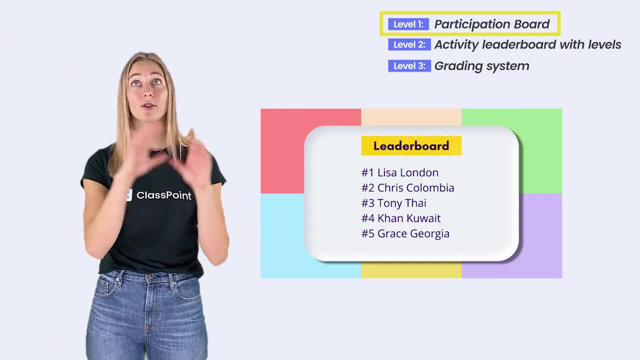 just be based off student participation, then totaled up and put into a leaderboard. You can display your leaderboard as a slide in your presentation with PowerPoint or Google. You can put it on your Google Classroom banner or, if you're in the physical classroom, just throw it. 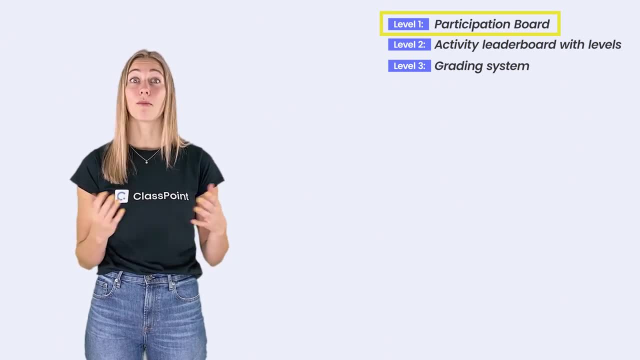 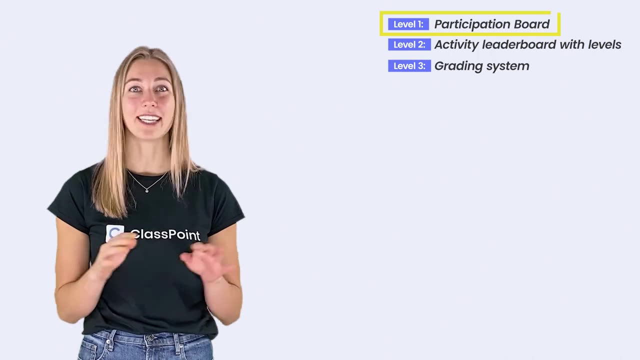 up on a bulletin board. If your classroom isn't really ready for the competition that leaderboards have, you can always assign code names to your students. That way their identity is hidden. Plus, it adds a little bit of intrigue and mystery. Take it up one level, because just participation. 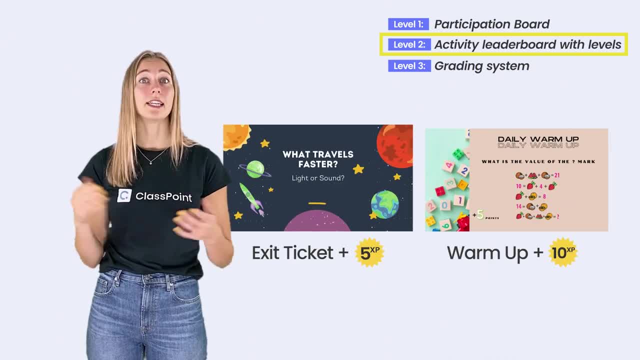 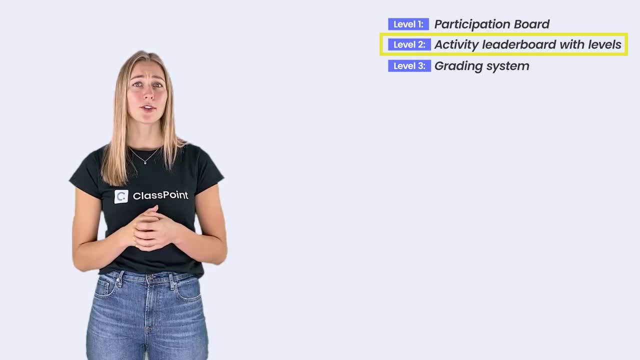 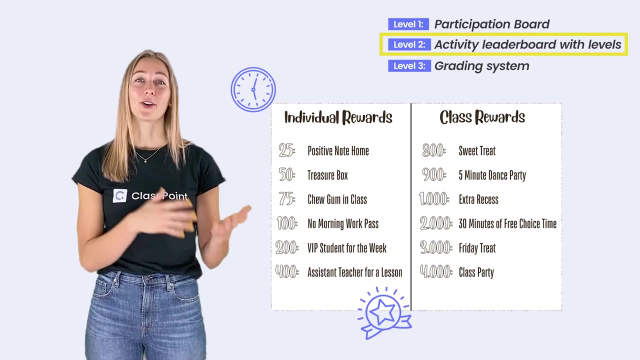 points is pretty minimum, So you can add in different activities throughout class for different opportunities for students to earn points, And then you can throw that up on the leaderboard as well, And once a certain number of points is accumulated, students can level up and get a reward. Rewards can be individual, like earning a free time or extra credit. 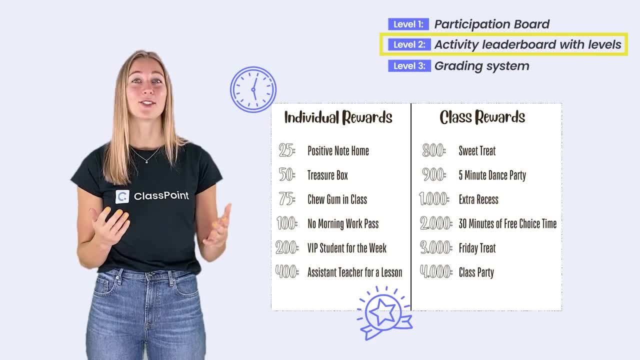 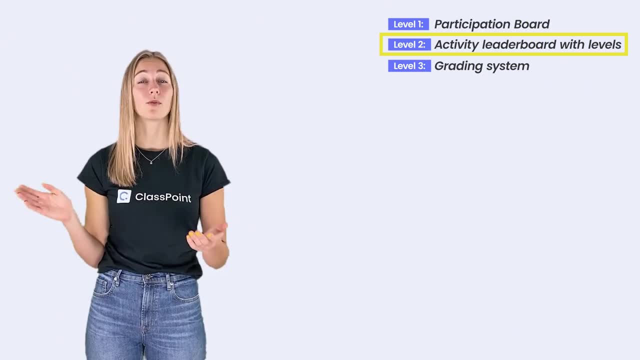 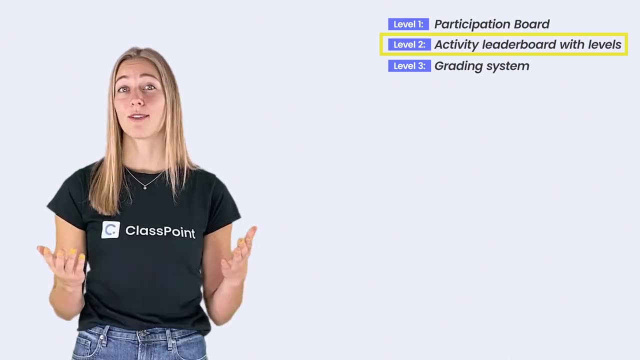 or students can pool their points together as a class to earn a dance party or maybe a pizza party. Providing students with the opportunity to have a lot of different ways to earn points is important, So make sure you have a variety of activities for students to earn these points, because every student can play the game a little. 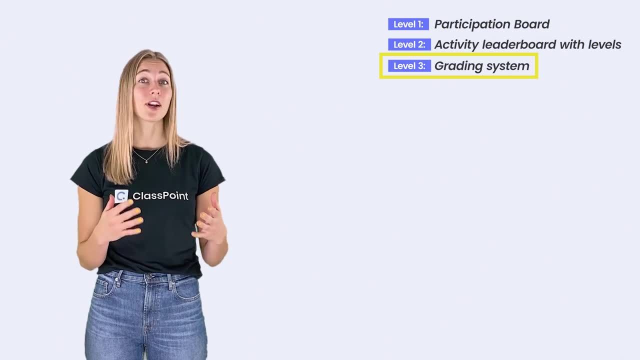 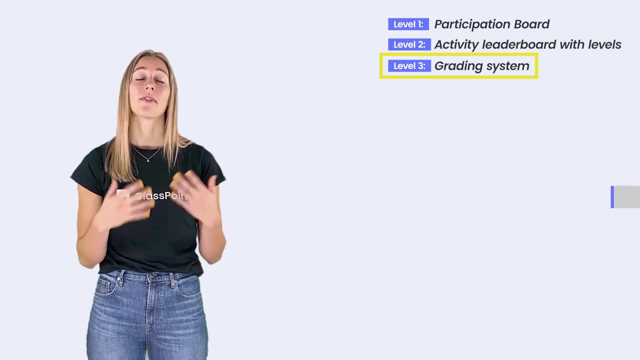 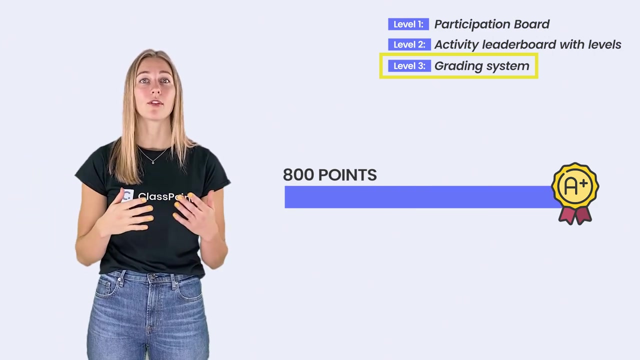 bit differently. Okay, now that third level, Turn all of these points into a grading system, So some teachers have actually used this point system as their grades. This way, it highlights the importance of progress and making sure that students are earning points towards an A instead of the look of every time having points. 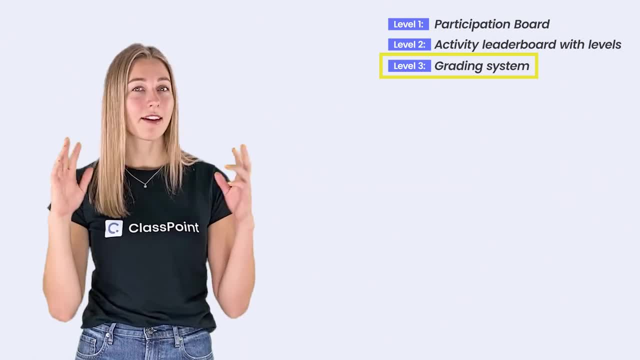 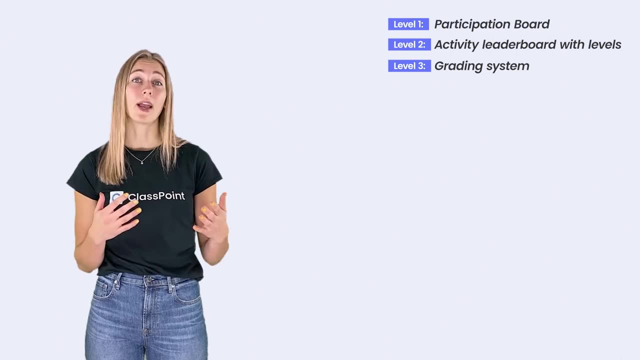 taken away and moving farther and farther away from an A. So it's just kind of a shift of perspective. Regardless of how far you want to lean into this classroom leaderboard, no matter what, it's a great way to get students motivated and involved in their own learning. 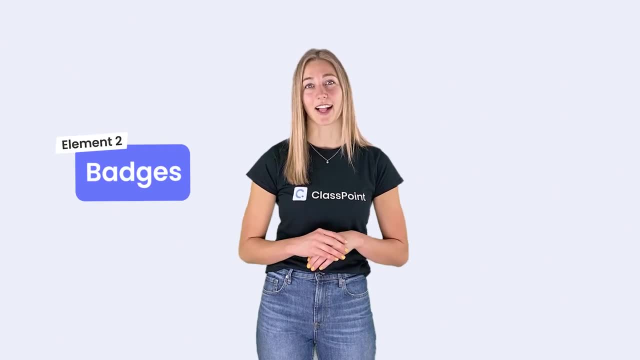 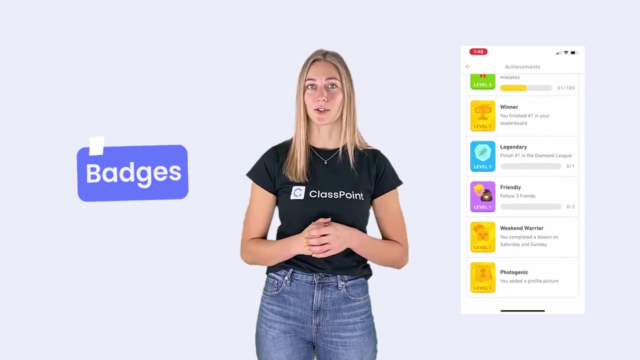 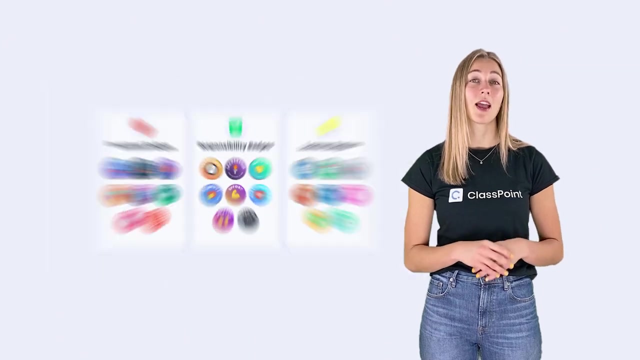 objectives. We can also add badge elements into the classroom. Many different games provide the opportunity for different levels or badges to be earned once a gamer masters the certain skill. In the same way we can incorporate that into the classroom to recognize students accomplishments and their mastery. So once students have mastered a certain skill or concept, 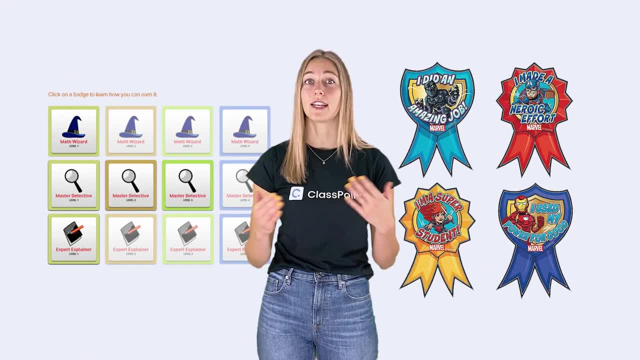 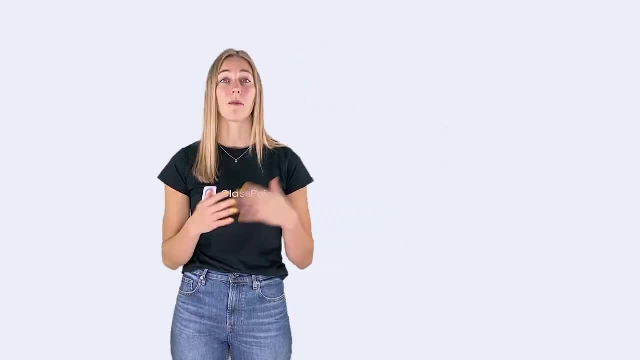 we can create and give them a new badge, or it can unlock the next badge or badge level. That way it shows that they have mastered that skill. These badges can then be displayed on a bulletin board or leaderboard. like we mentioned before, They can be combined with your point. 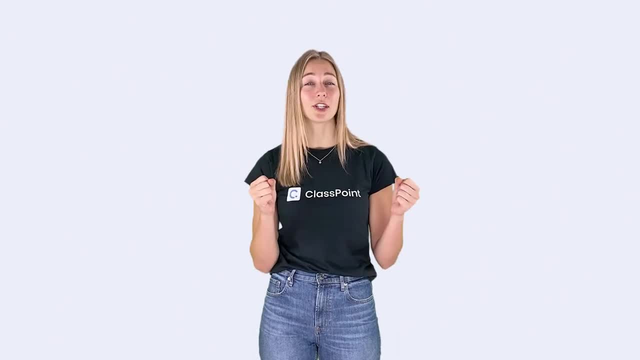 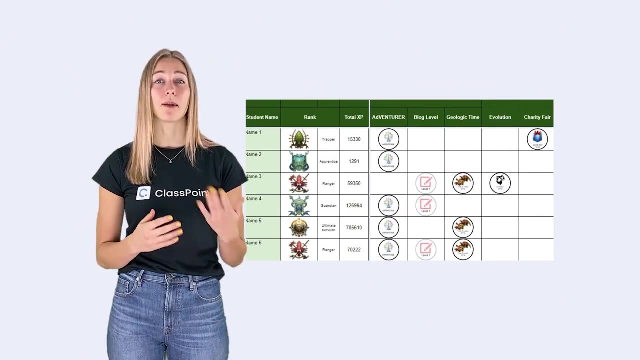 system leaderboard. That way everyone can see, everyone can cheer each other on, have a little bit of camaraderie or a little bit of competition. You can also give out these badges digitally and put them on students' profile on your LMS. Students can also help you to create. 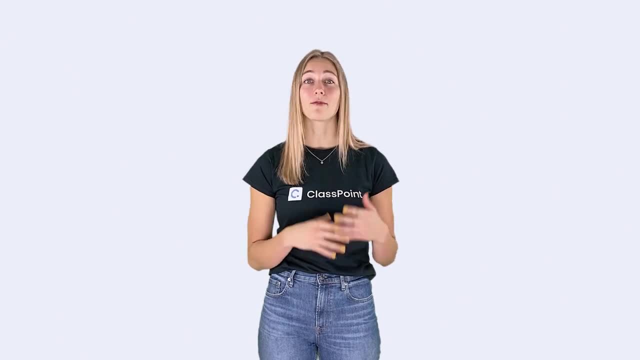 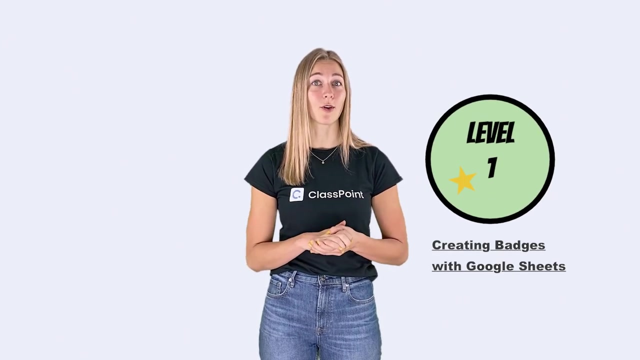 these badges. They often have a lot of good ideas, They're pretty creative and this gives them the opportunity to practice goal setting. Students can go ahead and create their badge, determine what is needed to earn that badge. Alice Keeler has a great short tutorial on how students can create. 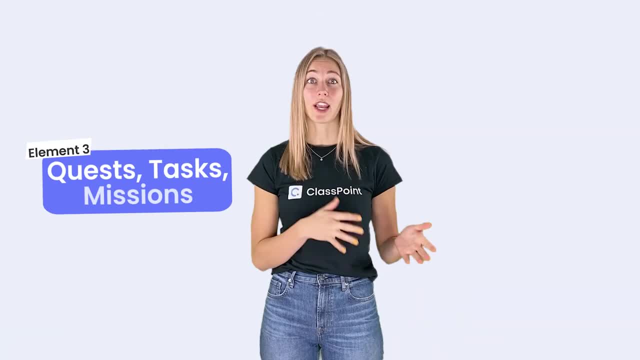 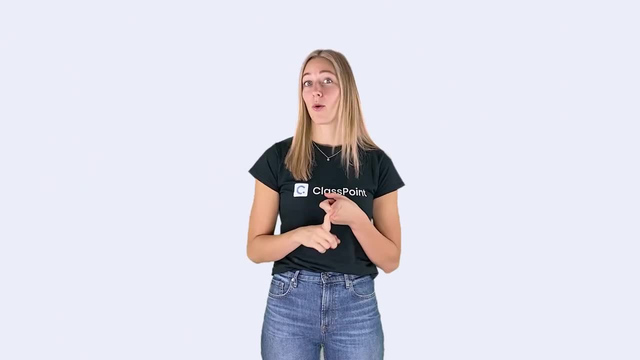 their own badges that I've linked in the description below. If you're interested, you can go ahead and click the link down below. Next, we can create quests or game-like tasks into the classroom. These are all really fun and there's lots of different ways that you can implement it. 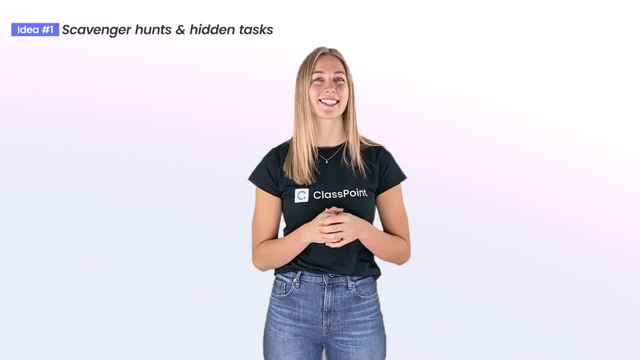 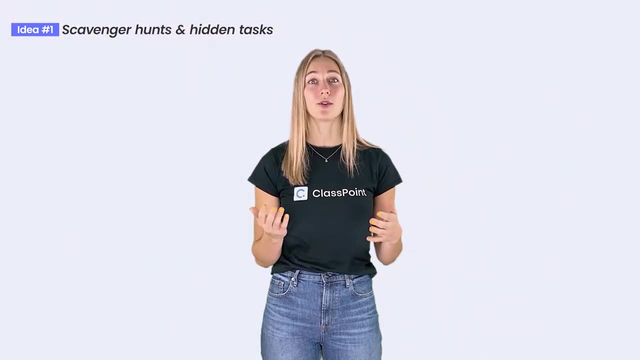 One idea is to do a scavenger hunt or a hidden task. Scavenger hunts are always really fun to add into the classroom and it's gamification already right there For this. you could use it as an assignment to have students search for a particular information in a reading. 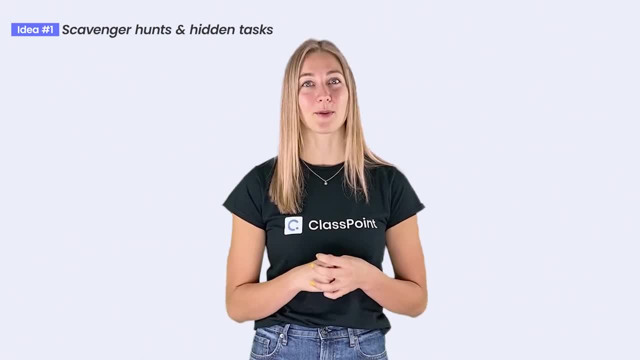 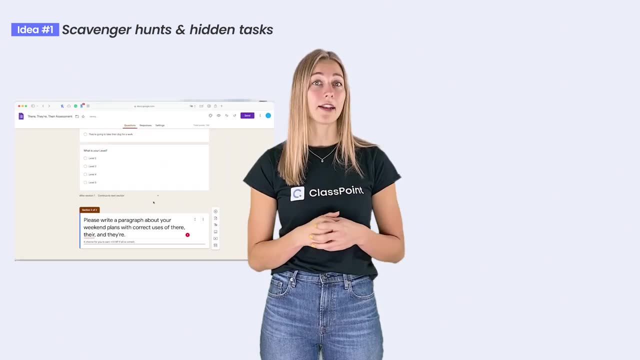 to make sure that they fully understand and they read what they were supposed to For these hidden tasks. let's say, if a certain achievement is made and students are on a level five, maybe at the end of a quiz there is a bonus question that can be unlocked for the level fivers. 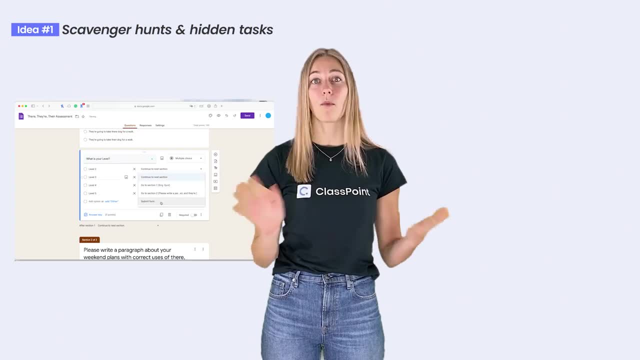 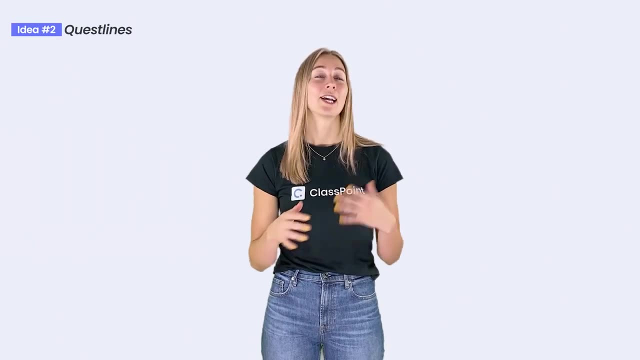 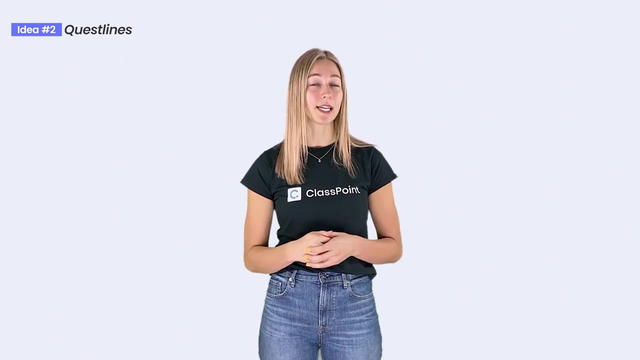 to answer and earn some bonus points. This can be done all right through a Google Forms with a password-protected question. Idea number two here is quest lines, Similar to a role-playing game, which allows gamers to choose their path and has different outcomes based on their choice. we can also give this opportunity to students to choose their path based on their choice. We can also give this opportunity to students to choose their path based on their choice. We can also give this opportunity to students to choose their path based on their choice. We can also give this. 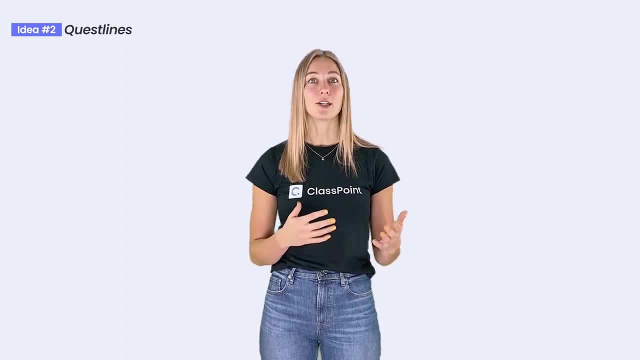 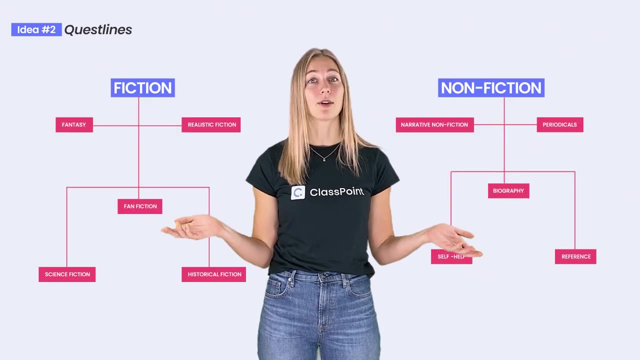 opportunity to students. For example, they can choose their own adventure for a book report. You can give them the option or the choice to choose fiction or nonfiction, and then broken down into genre and sub-genre. after that for them to choose. Idea number three: here is a current event task or 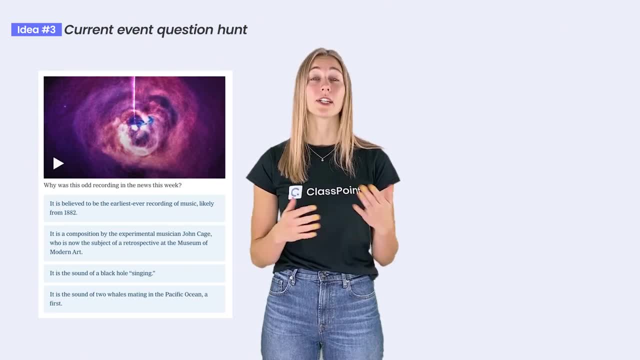 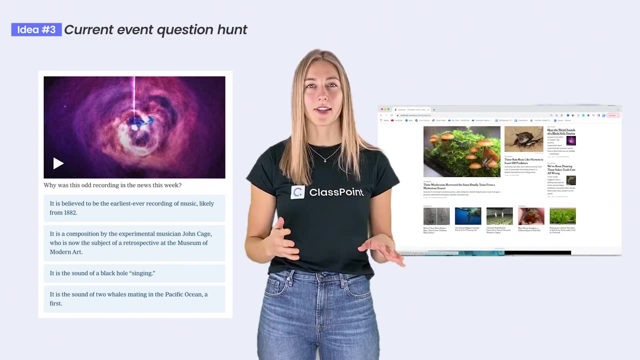 questions. Students can be on the hunt for particular information on a current event or something that's going on in your subject's community. Students are on this hunt because maybe every day you are on the hunt for a particular event or something that's going on in. 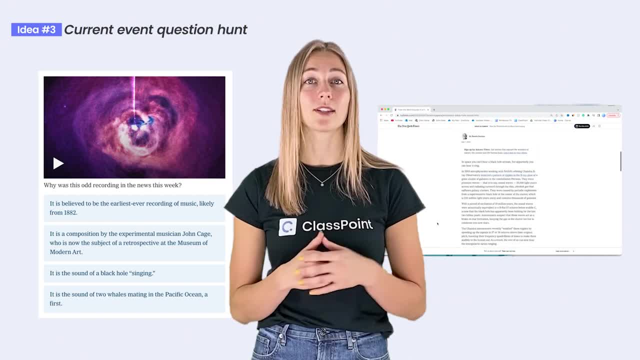 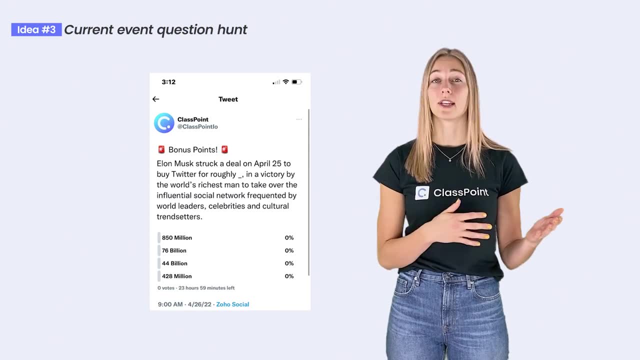 your subject's community. Maybe every day you ask a question on this topic so that students can earn a little bit of extra points. You can even add in bonus points or bonus questions to questions that you post in an LMS or on social media and if students answer those on those other sites. 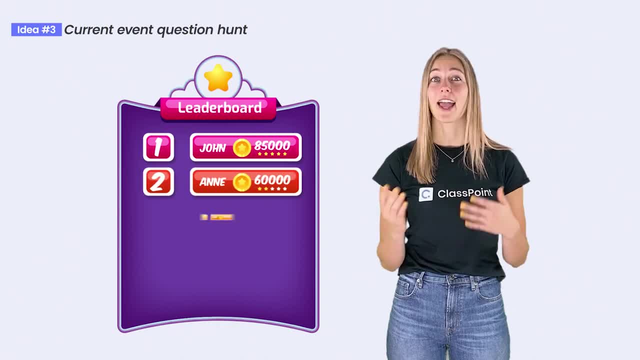 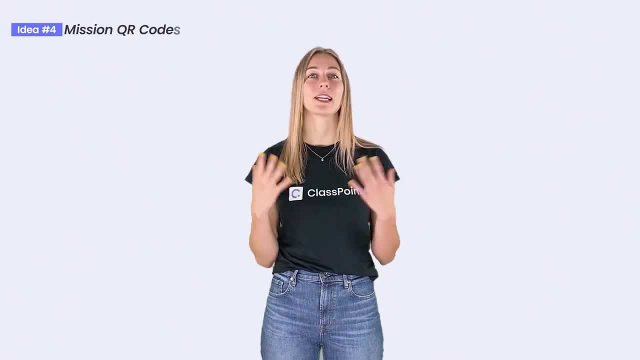 they can also earn some bonus points. Then at the end of your semester or the end of the year, the student with the highest amount of points can get a reward. Idea number four: here is mission QR codes So you can go ahead and place or. 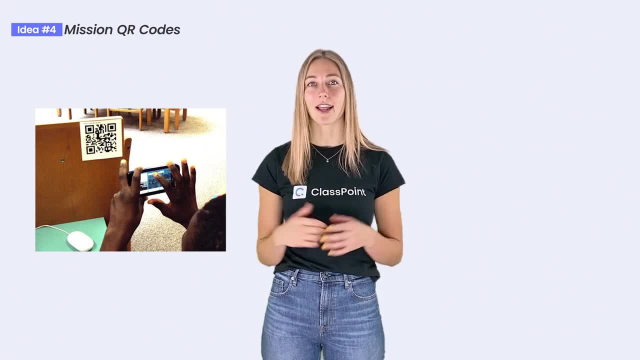 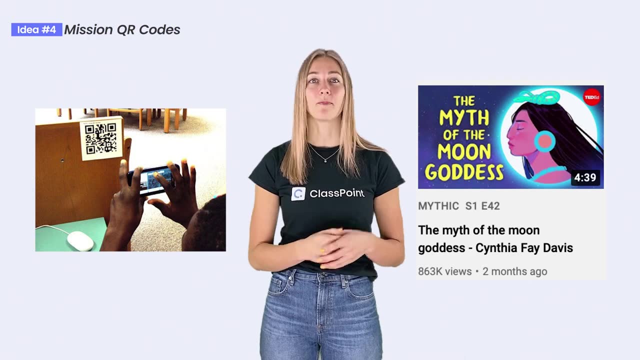 hide some QR codes around the school grounds to get students outside of the classroom learning a little bit or doing this learning when they're not in your classroom. It continues on that learning progress and every time they scan a QR code it's a different digital activity. 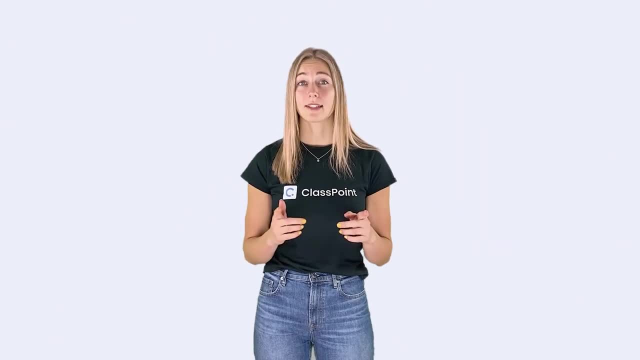 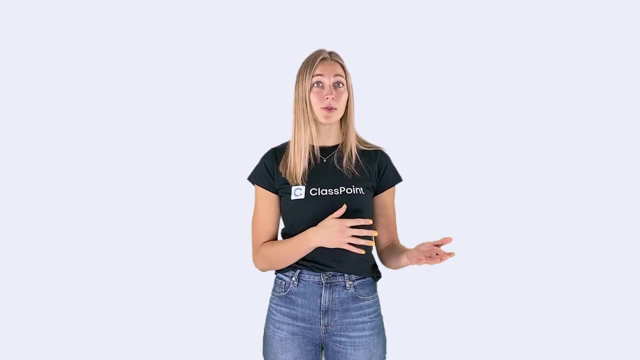 or game or something for them to learn. So you guys have to remember that we want these activities to be really fun but also doable for students. It's not going to have any effect if they're too simple and too easy and students get bored and don't want to do it, or they're too hard. 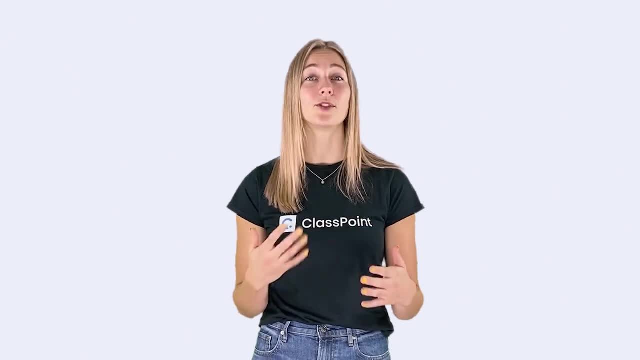 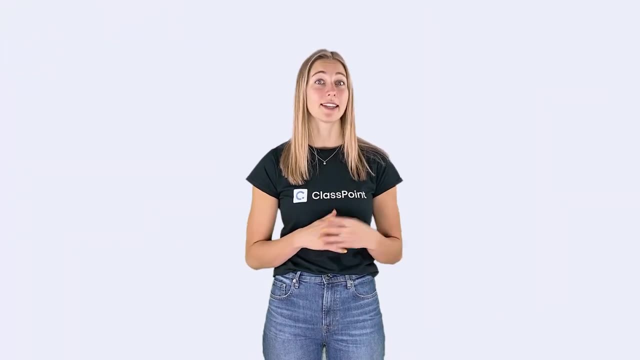 to even play in the first place. Our goal is to have students be inspired to take on a new challenge when they play these games and different activities. The last way that we have for you guys to add gamification into the classroom in this video today is with classic or digital games.